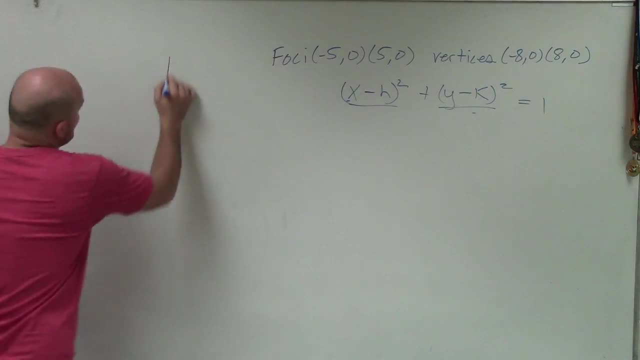 say: hey, just sketch it. Yeah, just draw what you have. There's nothing wrong with that, It's OK, We're just sketching the information we know. So they say the foci is negative: 5, 0.. 0, 1,, 2,, 3, 4, 5, 5, 0, 1,, 2,, 3, 4, 5.. And the vertices are negative: 8, 0, 1,, 2,, 3, 4,. 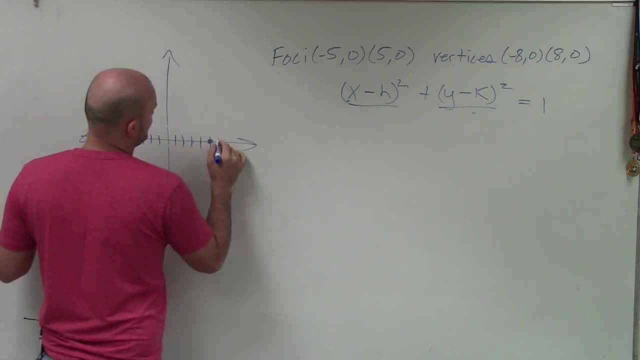 5,, 6,, 7,, 8,, 1,, 2,, 3,, 4,, 5,, 6,, 7, 8.. OK, Foci, foci, vertice, vertice. Now remember my conversation. 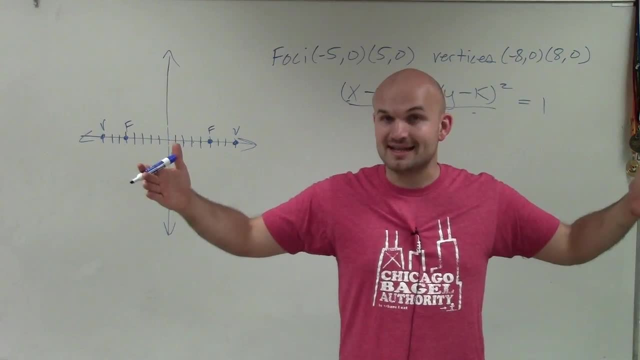 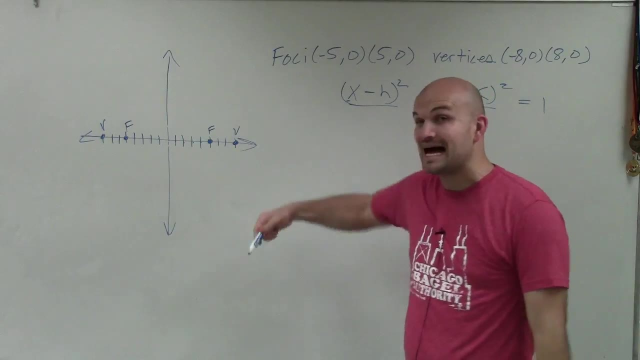 that I said. If the vertices are across from each other horizontally, then the a squared is under your x. If they're vertically, then the a squared is under your y. So we look at this and we say, all right, Remember, the vertices lie on the major axis, So it looks like my major axis is my x-axis. 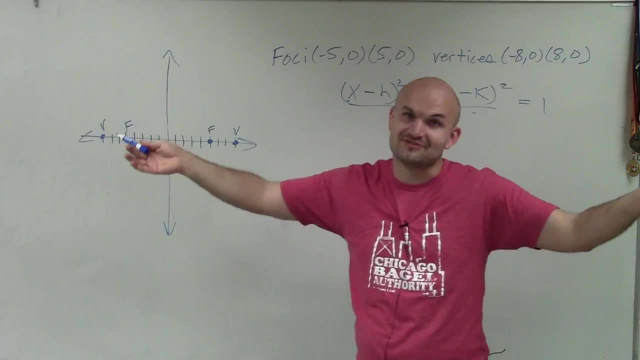 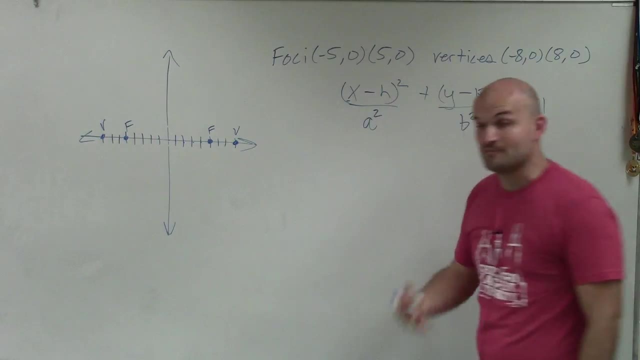 Is this a horizontal or is it vertical? Obviously it's horizontal, right, So we can say that my a squared is going to be under the x and my b squared is going to be under the y, where b squared, remember, represents the distance from the center to the co-vertice, which is 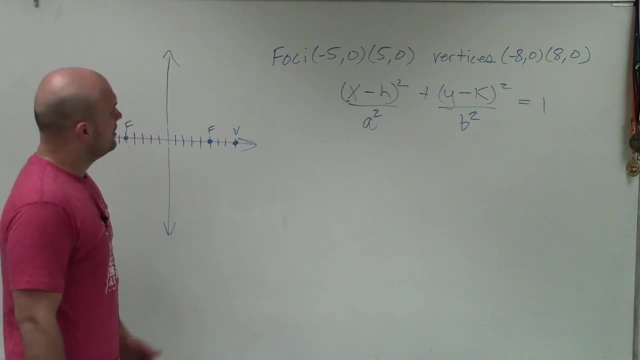 going to be up here or down. OK, So now we need to remember exactly what is a squared. a squared? All right, Let's see, Let's see, Let's see, Let's just deal with what a is a. oh well, first of all, all right, I kind of got ahead of myself. 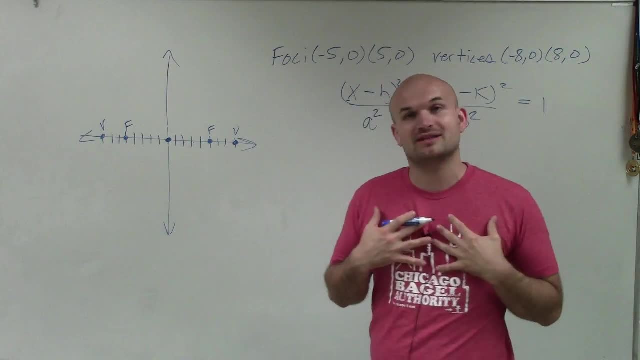 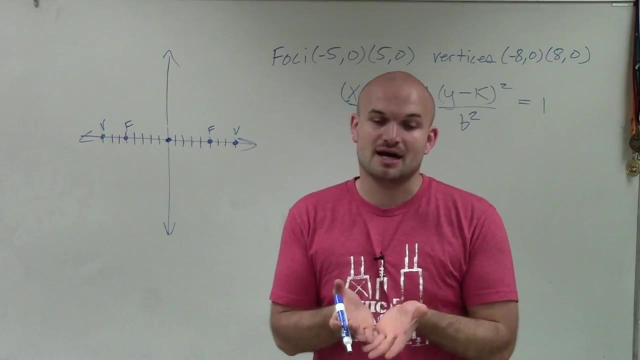 Sorry, I was talking a little too quickly. First let's find out what the center is. Now remember: the distance from the center to each vertice is exactly the same. The distance from the center to the foci to each foci is exactly the same. 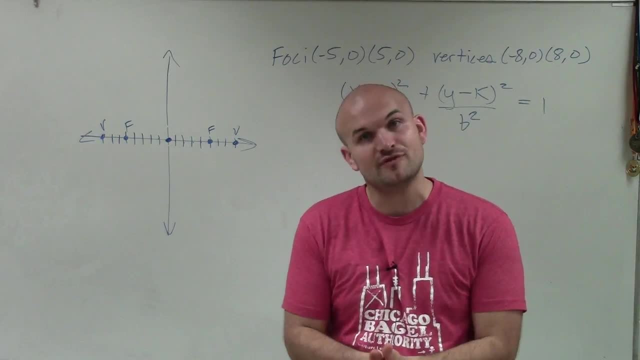 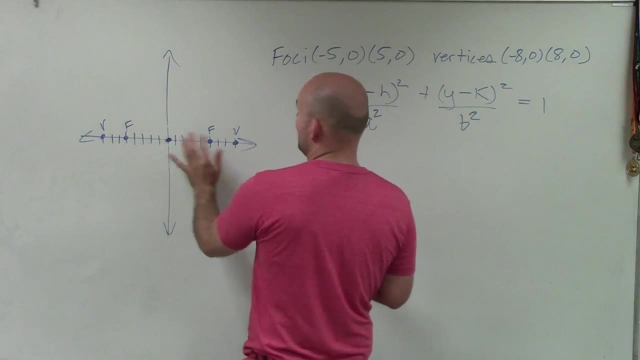 So, therefore, the center is going to lie directly in between the two foci, as well as the two vertices. So you can see that, since this is 8 in both directions and this is 5 in both directions, you can see that my center is at 0, 0.. 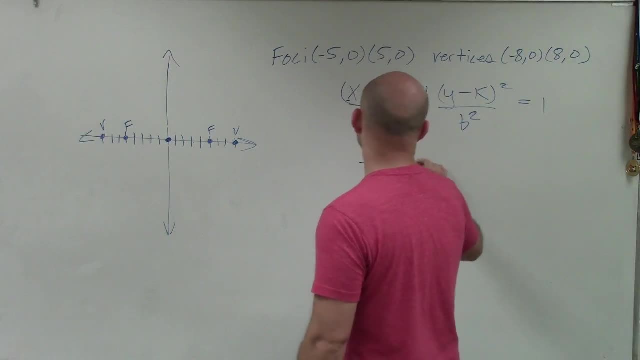 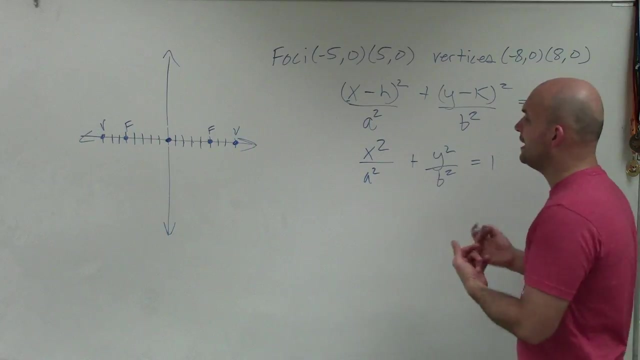 So therefore, I'm going to change my equation to: x squared over a squared, plus y squared over b squared, equals 1.. There's no h and k. Well, there are. The h and k are both 0.. So we can just write them as x squared and y squared. 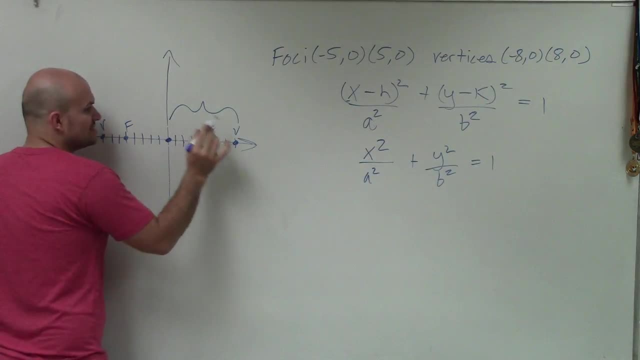 So again, the distance a is the distance from the center to your vertice, that absolute distance which is a. Well, a equals 8.. The absolute distance from your center to your foci is going to be b, which, in this, 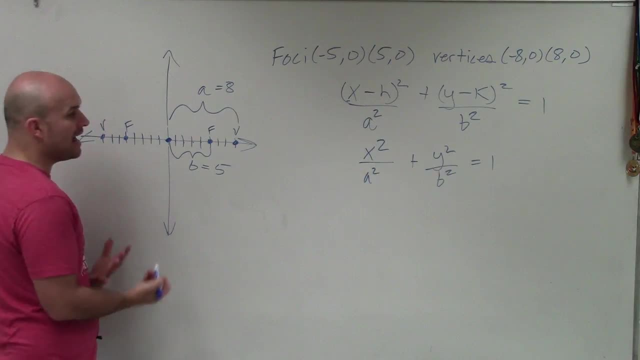 case is 5.. So now I can. I'm sorry, that is c, I'm getting. ah, I'm getting ahead of myself. So that is c. The next thing now is we still need to figure out what b is. 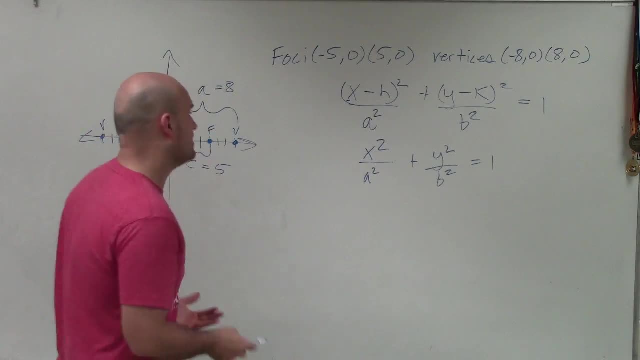 So again, if you remember, when we were working on graphing them, one thing to find out what a lot of times what c would be, we'd have: c squared equals a squared minus 1.. So that's a squared minus 1.. 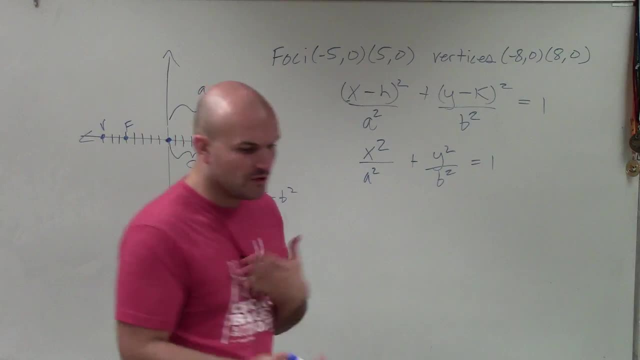 So that's a squared minus 1.. That's b squared. This is how the, this is how your foci, your vertices and your center all relate to each other. So I know what c squared is: That's 25.. 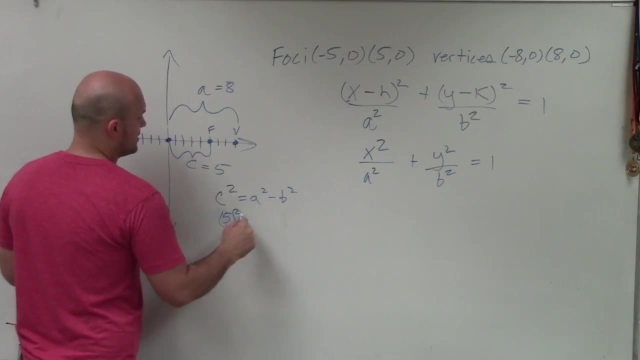 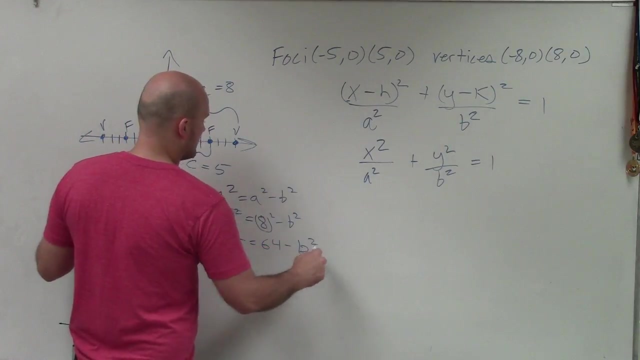 Ah, let's write it in there actually. So I know, c is 5 squared equals a squared minus b squared. So 25, 5 squared is 25 equals 64 minus b squared. All right, So now what I can do is just subtract. 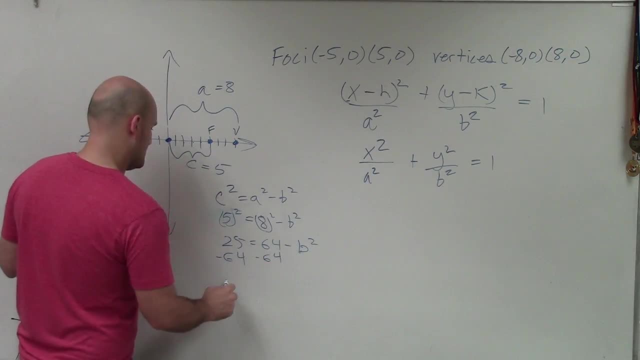 64 on both sides And what I can have is a negative. ah, bup, bup, bup 81, what am I doing? That's a negative 81.. That's going to give me a negative 41 equals negative b squared. 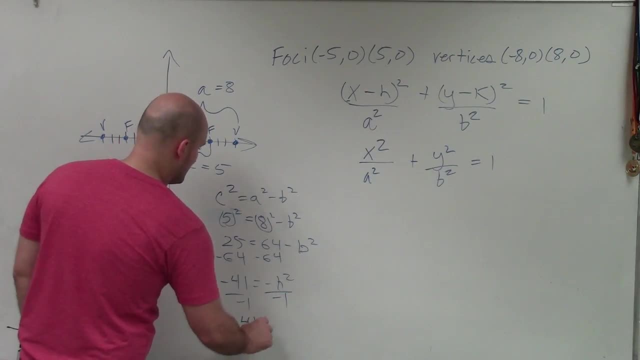 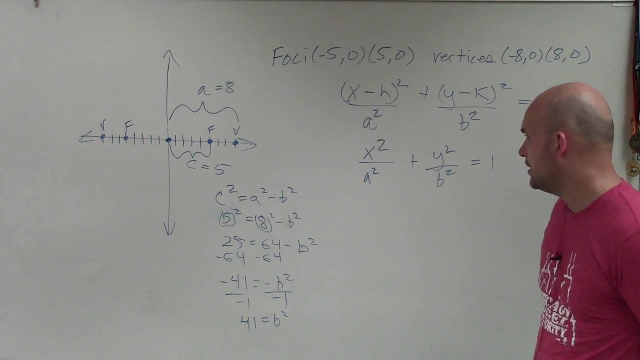 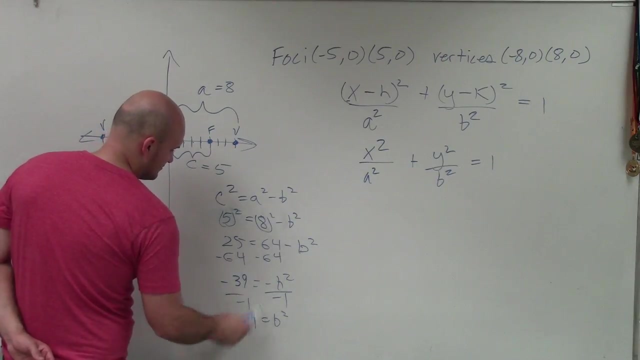 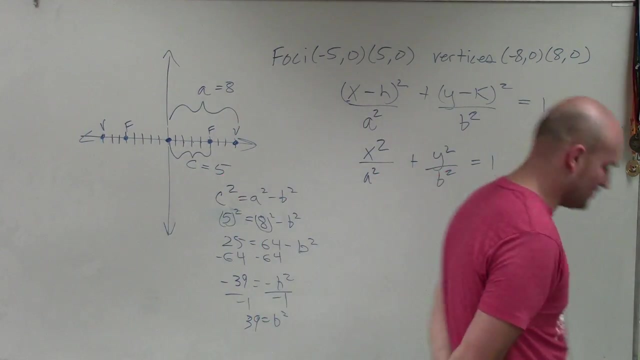 Then I divide by negative 1.. Divide by negative 1.. I have 41 equals b squared. No, That's going to be a 39.. What am I doing? There we go? 39,, 50,, 64.. 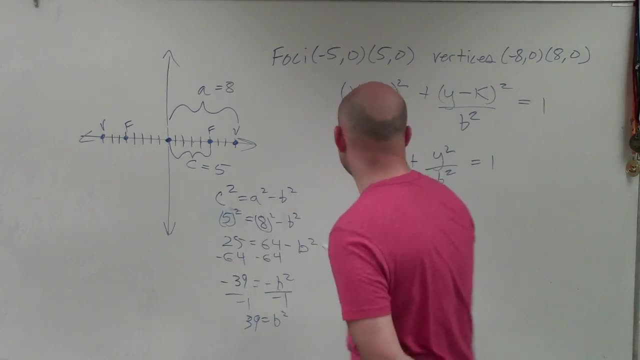 There we go, Okay, So now it's going to be 39.. So that's going to be my b squared, which I don't need to solve for b. I can just plug that in. So I know a squared, Ah. 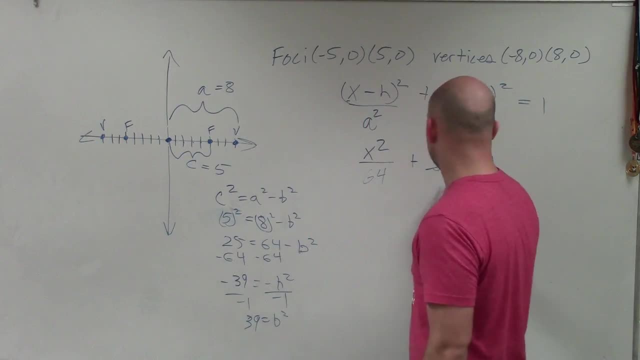 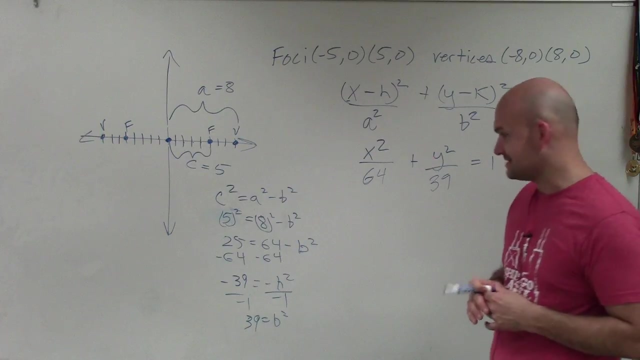 Ah, That is 64 plus b, squared is going to be 39.. And there you go, ladies and gentlemen. That is how you write it into your standard form. Thanks,